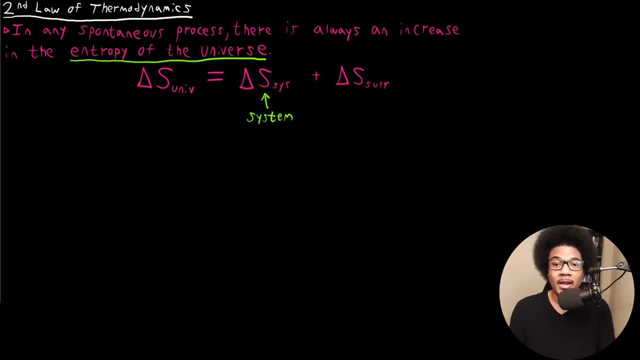 whatever thing you're studying is going to be equal to the changes in entropy of the system and the surroundings. So you're going to describe thermodynamically whether it's a chemical reaction or a gas sample or what have you, And then this is the change in the entropy. 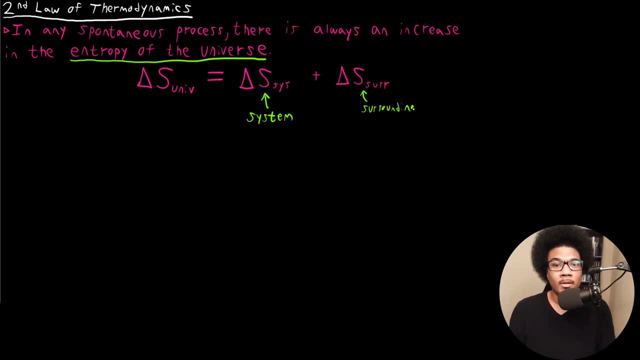 of your surroundings, right, And the sum of those gives you the change in entropy of the universe, right. So, basically what this says, right, If, if the second law of thermodynamics, if we take this statement right, basically what we're saying, is that a positive change? 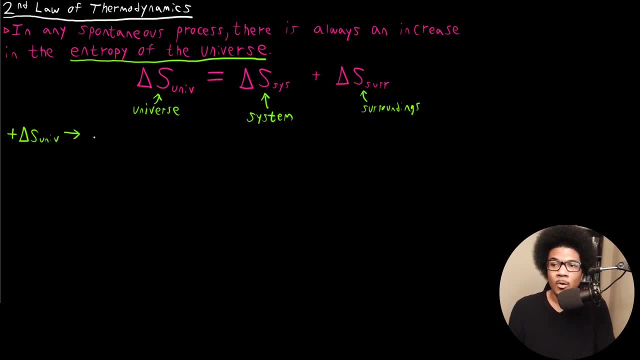 in the entropy of the universe corresponds to a spontaneous process, right? Whereas a decrease in the entropy of the universe corresponds to a non-spontaneous process, right. Or if it's, uh, if it's a process that can be reversed, then you can say that it's. 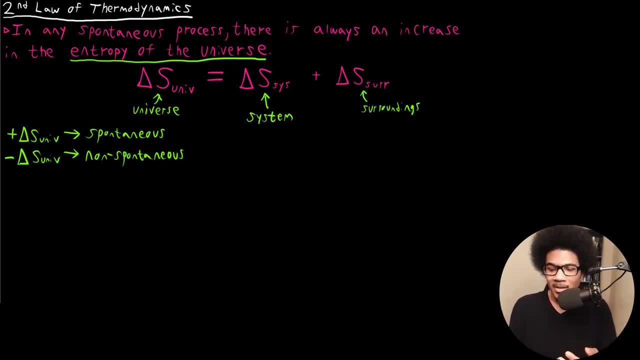 spontaneous in the reverse direction If you have a negative Delta S of the universe, right Okay. So let's see how we can actually uh, how we can actually identify whether uh a process is going to be uh spontaneous or not. 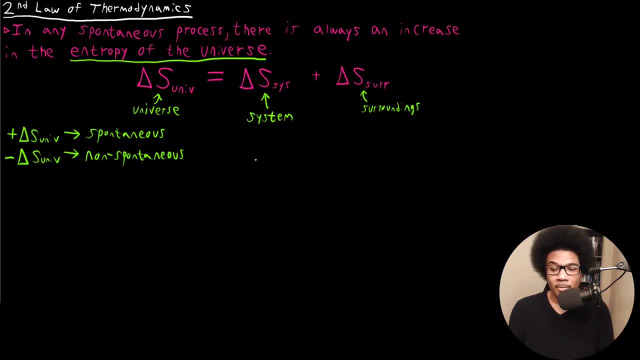 right? Um, so let's see. So let's, let's map out our thermodynamic system. So let's say, we have some system and I'll use a different color here. Let's say, we've got some system here, Let me might make that a little bit smaller, right? So this is our system. 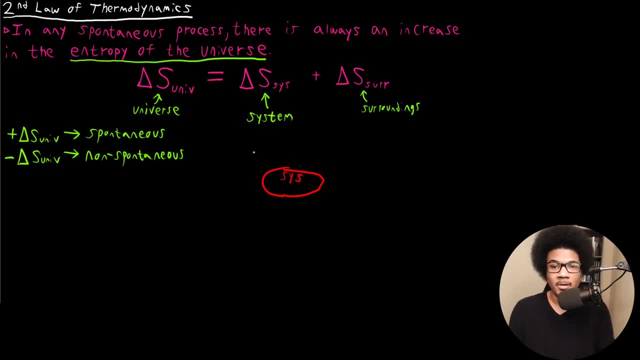 right, We've got our system here. I'll put S Y S there for system and everything on the on the outside of it is our surroundings, So I'll use a dotted circle here for the surroundings, right? So we've got our system and our surroundings. 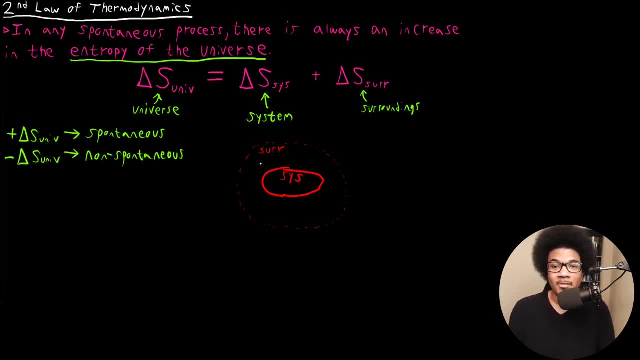 Let's say that we have heat flowing from our system to the surroundings, right? So I'm gonna draw an arrow here and keep in mind that heat is denoted by the lowercase Q for heat. So heat is flowing from the surroundings to the system. 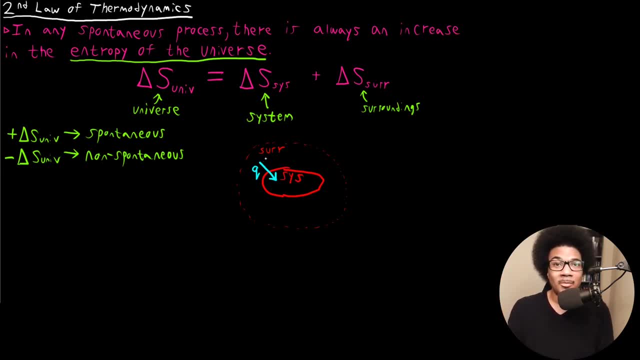 So I ask you um figure out whether this is spontaneous or not. Do we know whether this is spontaneous or not? Well, no, we can't really figure out, just from knowing the direction of the heat flow, whether the system is, whether this is going to be a spontaneous process or not, right? So? 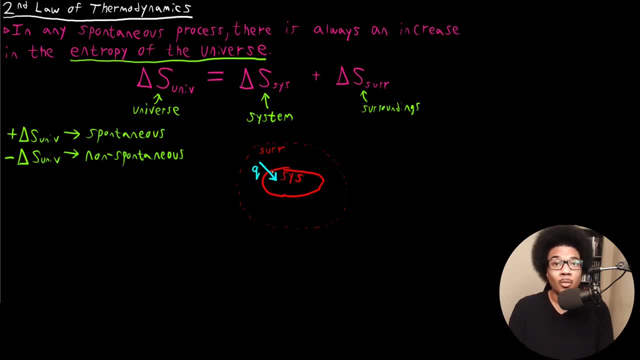 keep in mind, we talked about enthalpy, right. All you need to know was whether heat was flowing from the system or into the system in order to figure out whether something was endothermic or exothermic. But here we can see it's a little bit more uh. 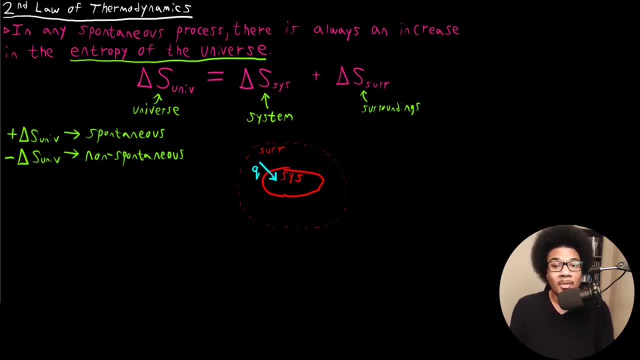 robust because we have to know the magnitude of the change in heat from the surrounding to the system, or else we can't really say whether this is spontaneous or not. I mean, there might be a increase in entropy of the system, but you know how great is that change? Is it enough to overcome? 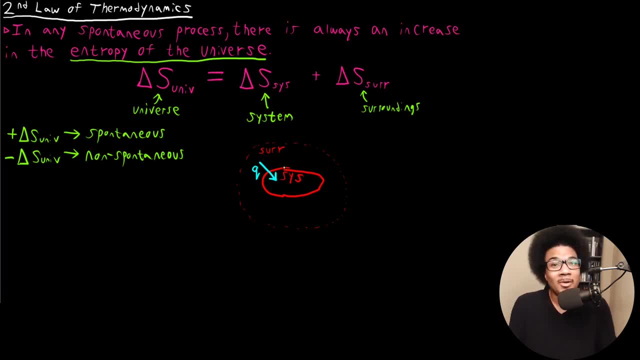 the, the loss in entropy of the surroundings, You know it's, it's going to be dependent on the magnitude of all of these things. So what I want to do is put a little bit more specificity into this, right. So I'm going to draw a second thermodynamic system here, right, Just like the? 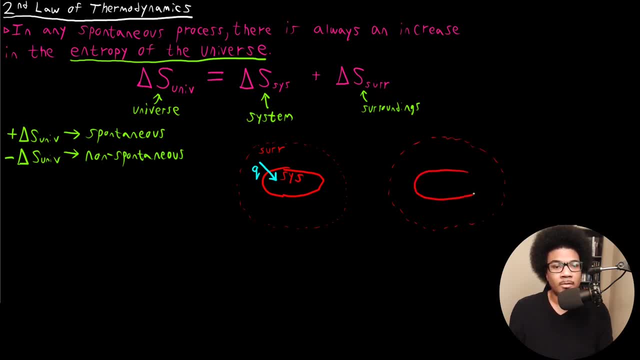 first I'll use a dotted circle for the surroundings, solid circle for the system, right? So we got two different thermodynamic systems. Let's label them both. We got: we'll call this guy system A, we'll call this guy system B. In both cases we're going to have heat. 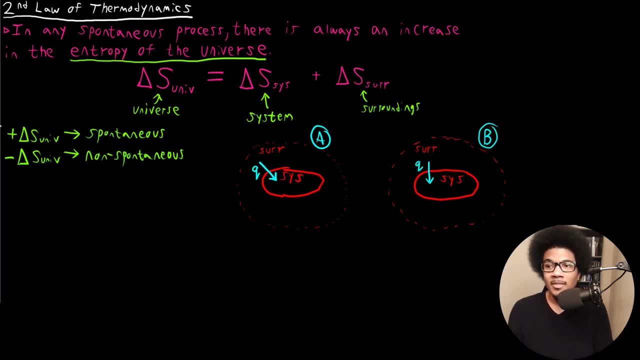 flowing from the surroundings to the system. right, And in fact it's going to be a little bit more the exact same quantity of heat that's flowing from the surroundings to the system. However, I'm going to have each of these, each of the surroundings, at two different temperatures. 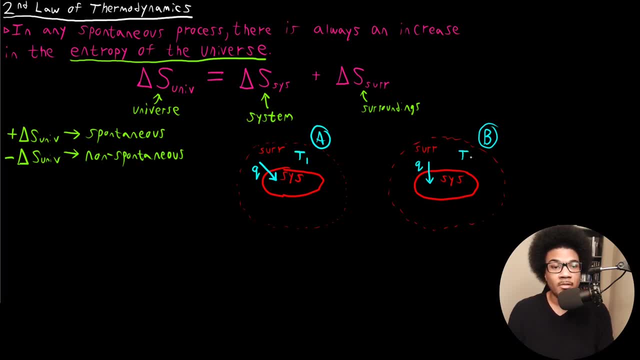 right, So we'll have T1 and T2, right? So we got a temperature T1 and a temperature T2 for our surroundings, And what I'm going to say here is that T1 is going to be much, much greater than T2, right So? 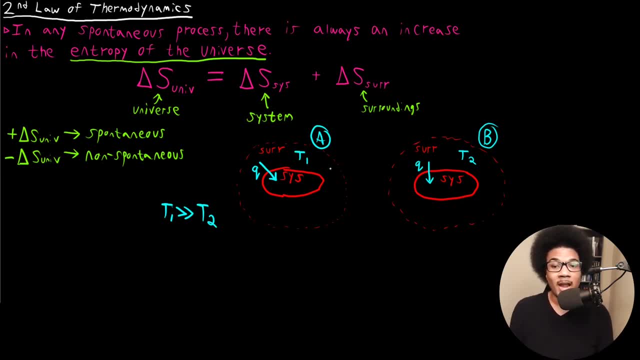 this is what we'll set up for the comparison of these systems. They're at two different temperatures and the temperature in the surroundings in system A is going to be much, much greater than the temperature two here in system B right Now. Q is going to be the same in both cases. Let me 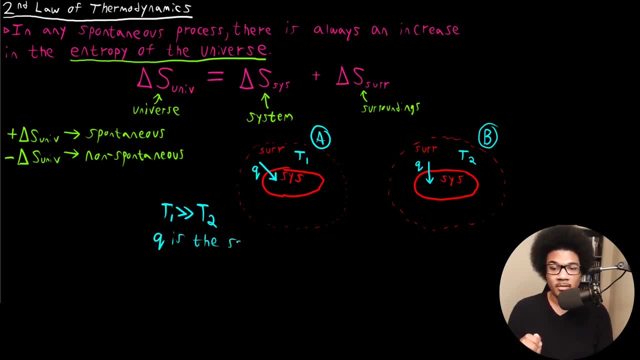 write that down. So Q is the same in both cases, right. So the same exact magnitude of heat is transferred from the surroundings to the system. So so now the question is which one is going to have a greater change in the delta S of the surroundings? right, In which one would the? 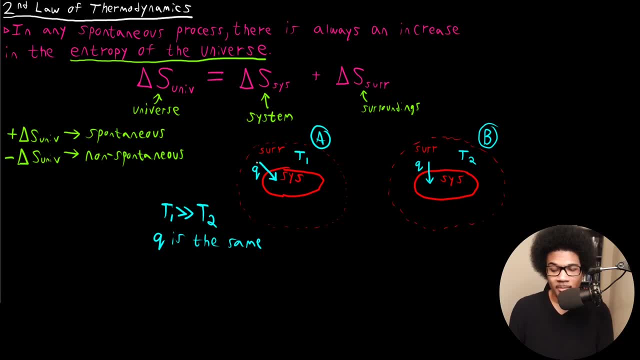 disorder decrease the most right? So, in order to answer this question right, we have to figure out which one of these temperatures is greater. We know that it's temperature one, So that means that the magnitude of the change in the surroundings is actually going to be much greater in temperature. 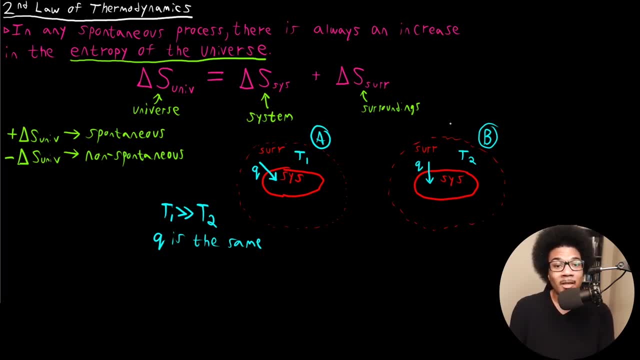 two, since it's the lower temperature. So the magnitude of delta S of the surroundings is going to be much greater in system B than it would be in system A, because it had less thermal energy to begin with. right, So it's giving a. 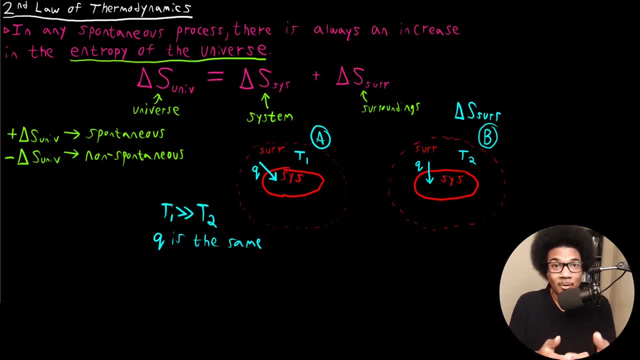 certain amount of heat, but it had less thermal energy to give in the first place, So that's going to have a much greater effect on its entropy. So the example that I like to use in this case is: you have two friends and you ask both of those friends for $10, right? And your first friend is: 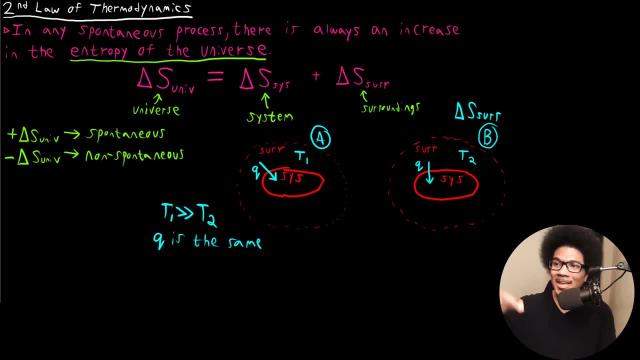 rich. Let's say he has $5,000, right To his name And he gives you $10, right. But your other friend only has $15, but he also gives you the $10, right. Which one is it going to mean more to you? 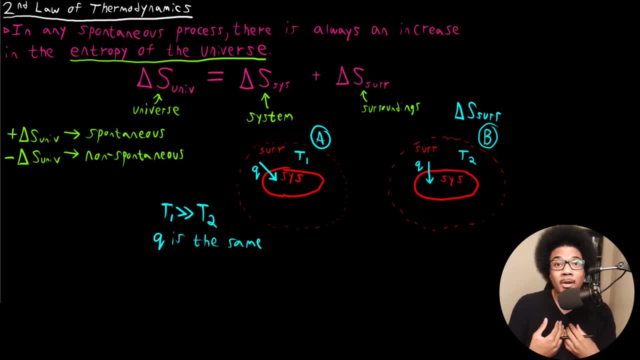 I mean, either way, you're getting 20 bucks, right, You're getting the same amount of money, but it's going to mean a little bit more coming from your friend that only had $15, right, $15 to his name- versus your friend that had $5,000, because you know it's going to have a 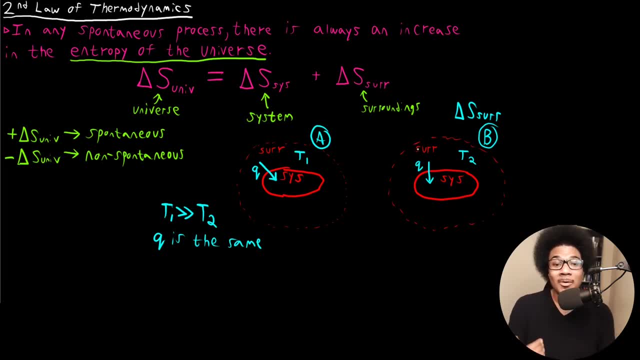 bigger impact on his finances, right? Same type of deal here, where if the surroundings has less thermal energy to give in the first place, it's going to have a greater effect on his entropy to give the same amount of heat, right? So keep that analogy in mind when you're thinking about. 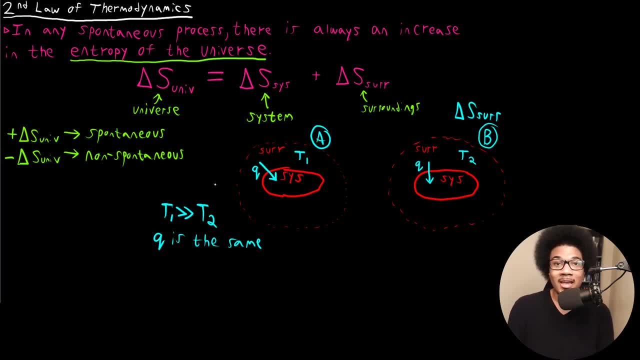 the magnitude of Delta S in these cases. If there's a less amount of thermal energy here to begin with, then it's going to be a little bit more impactful on the entropy of the system. Okay, So we see here that it not only depends. 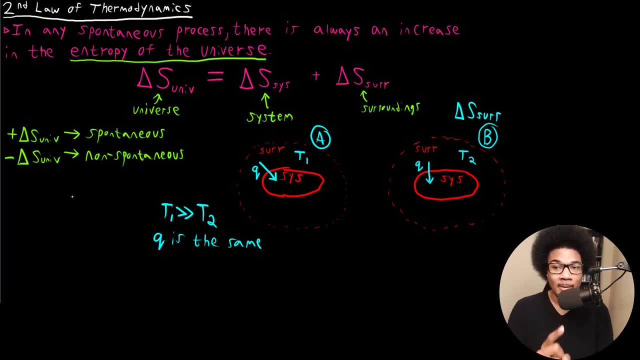 on the amount of heat transferred. It also depends on the temperature how we calculate Delta S. So that leads us to an equation. So if we want to calculate the entropy change in the surroundings, right, So if we want to calculate Delta S of the surroundings, 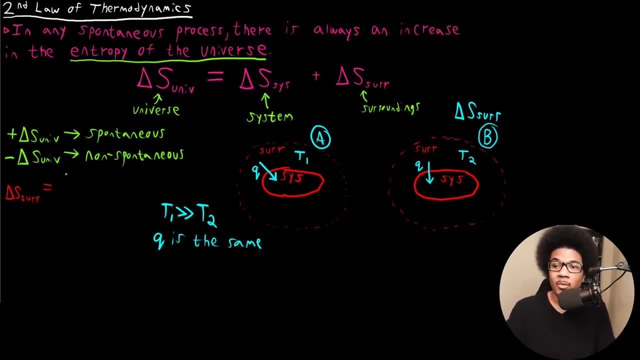 right, We're going to have a ratio between the quantity of heat released by the system, right? So I'll say quantity of heat, And this is typically in joules, but it can be in kilojoules or whatever energy value that you're. 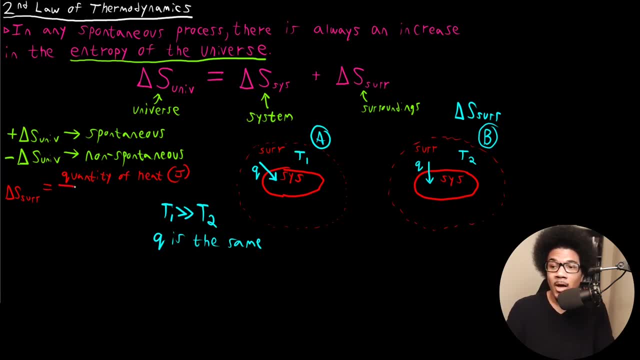 using to quantify your transfer of heat. So the quantity of heat that's released by the system over the temperature, right, The temperature of your surroundings, Right? So we have this ratio between the energy transferred and the amount of the temperature of your surroundings, right? So- and I kind of mentioned this in the previous course, 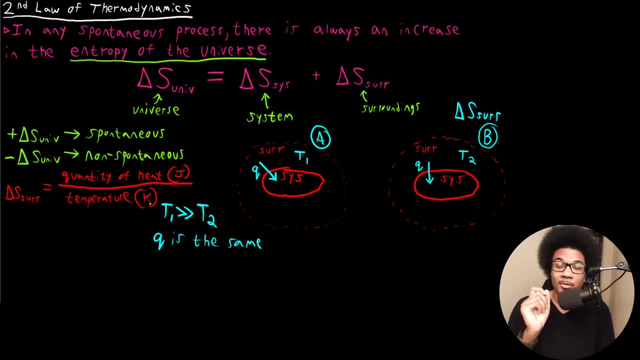 but I want to reiterate this here- that you always want to make sure you're using the absolute temperature, the Kelvin scale, when you're doing these calculations. If you use Celsius or Fahrenheit, you might get erroneous, negative values that will throw off your 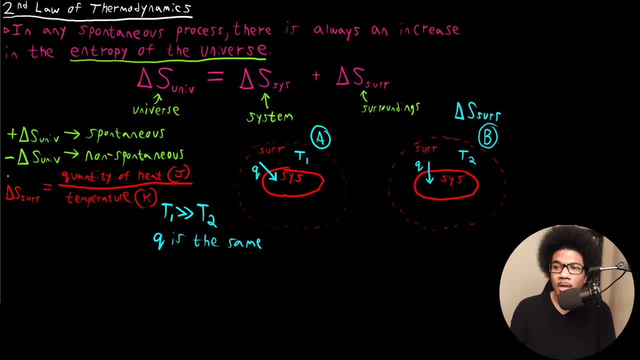 interpretation of the change of the entropy. Okay, So you know, we have this ratio between the energy. to write this as an equation? right, I'm going to write the equation for the delta S of the surroundings. The equation is going to be negative And I'll talk about that negative sign in just a. 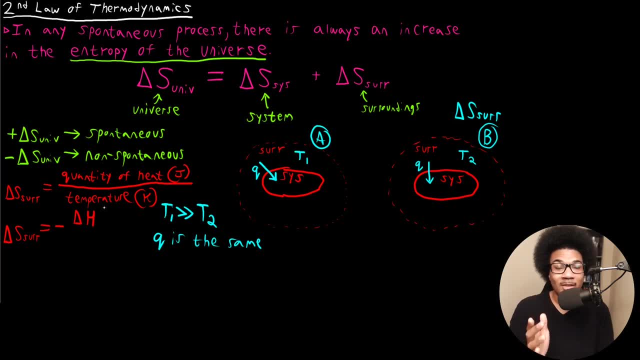 second, right Negative delta H. right Delta H is our change in enthalpy. right That we talked about this in a previous course, where this is a thermodynamic variable that's used to quantify the amount of heat that's being transferred in a system. right, So we have, we can use that here. 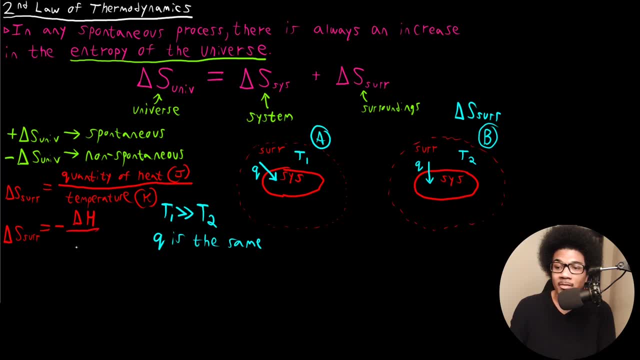 to quantify the amount of heat transferred. That's going to be over the temperature, right? So this would be our equation to calculate delta S of the surroundings, right? So now about this negative sign. So this is just to maintain our sign convention here, right? So we know that if 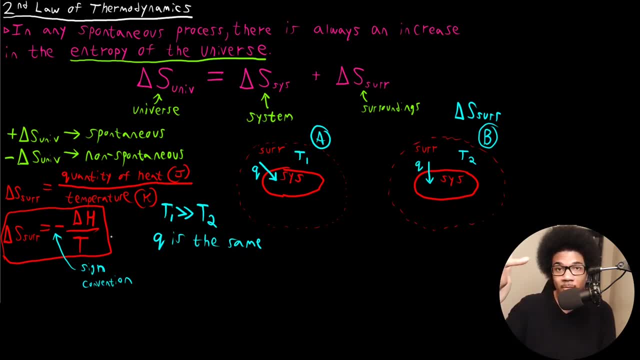 heat is transferred from the system to the surroundings, that's going to increase the entropy, the surroundings, right. But we know that if heat is released by the system, it's going to give a negative enthalpy value, right? So if that enthalpy value is negative, this negative sign just ensures